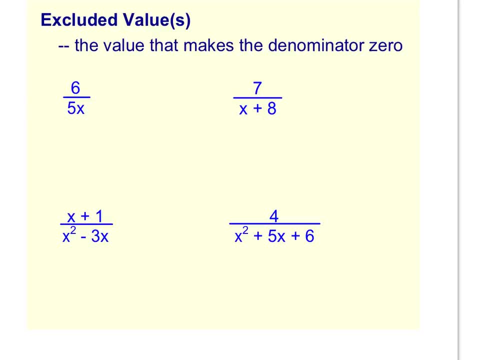 To find the excluded value. we want to remember what excluded values actually are, So I just threw the definition up here. It's the value that's going to make the denominator equal to zero. If you remember, in math that's the one number you can never divide by. 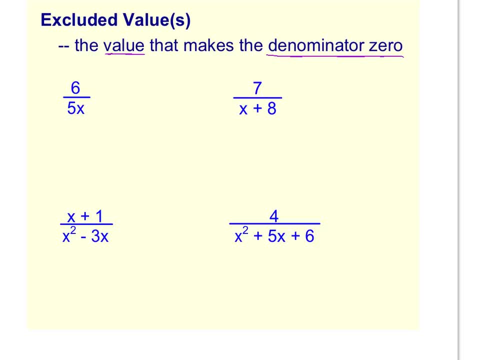 Anything divided by zero is undefined, So we try to avoid having that happen. So if you're asked to find the excluded value, here's all you have to do. You look at your denominator, grab the denominator, write it out here. We know that that denominator 5x cannot equal zero. 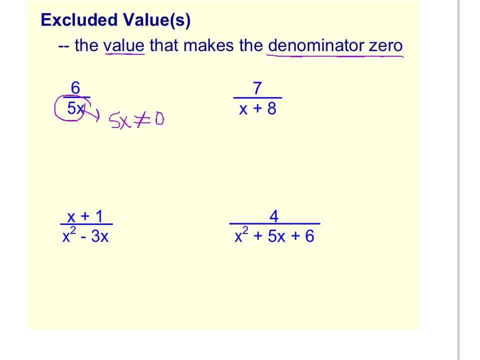 Once you have that statement then it's as easy as solving for x. You know, in this case we would divide by 5. So we have x cannot equal zero And that is our excluded value for that first rational function. And if you think about what would happen if you plugged a zero back in for x, right here, 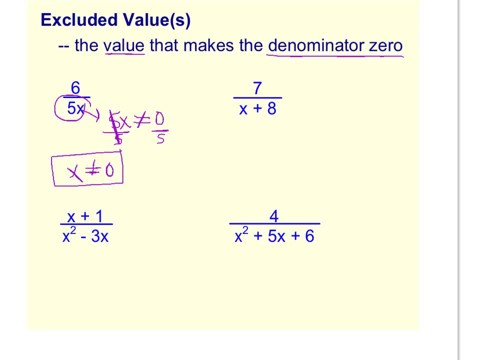 Well, 5 times zero is zero, And 6 divided by zero is undefined. So zero is the value that we have to exclude for x. Alright, so again, our next example: to find the excluded value, just grab your denominator. 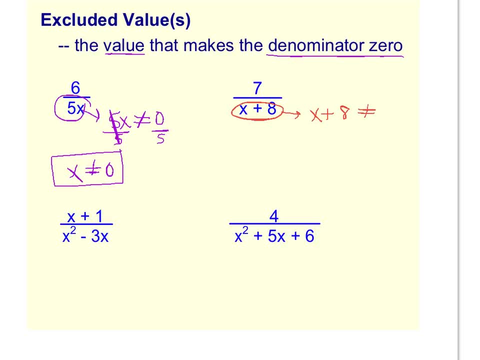 Go ahead and say that x plus 8 cannot equal zero And then solve for x. So we'll subtract 8 from both sides. So x cannot equal a negative. And again, if you look at you know the problem. if you put a negative 8 in for this x. 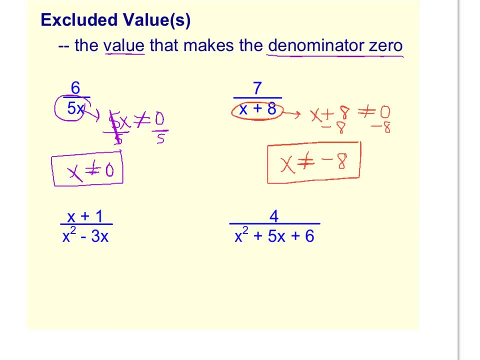 negative 8 plus 8 equals zero. 7 divided by zero is undefined, So we will exclude negative 8 from all the values that x can equal. Alright, so those two are pretty basic and straightforward. Sometimes you can come up with a number just by looking at it. 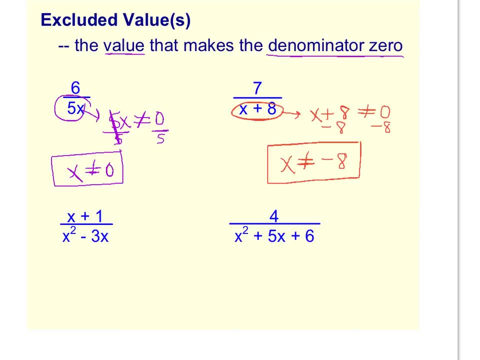 But again, taking the denominator out. that's something you can do on every single example. Okay, Okay, Okay, Okay. So, for example, this next one: if you grab the denominator and say, alright, x squared, oops, not plus x squared minus minus 3x cannot equal zero. 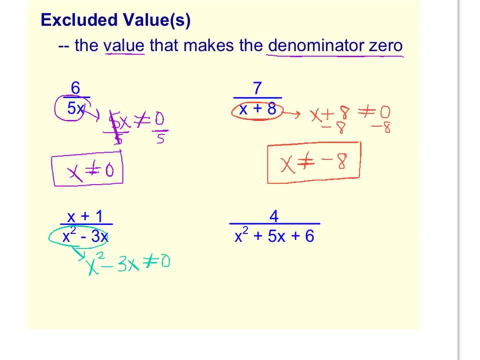 So for this whole chapter on rational functions or rational expressions when in doubt factor everything. Because of the x squared and the 3x, you have x's in two spots. you cannot just solve for x like you normally would. So for this whole chapter on rational functions or rational expressions when in doubt factor everything. 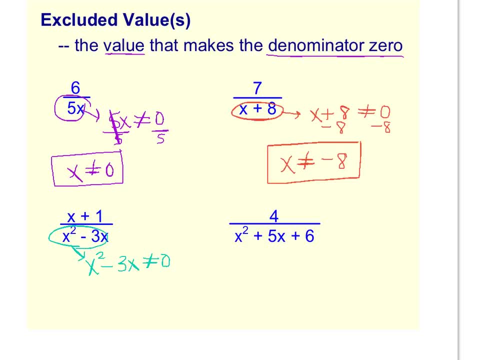 Because of the x squared and the 3x, you cannot just solve for x like you normally would Like the examples above. We have to actually factor this out. So wherever you see it, so factor out. think about, in this case, GCF. 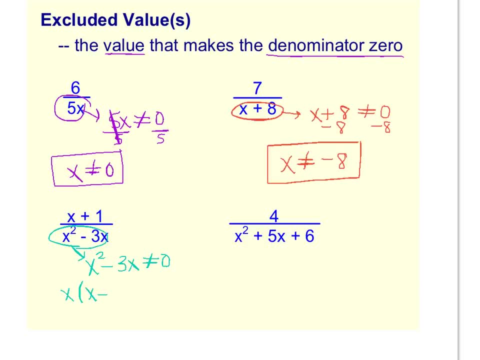 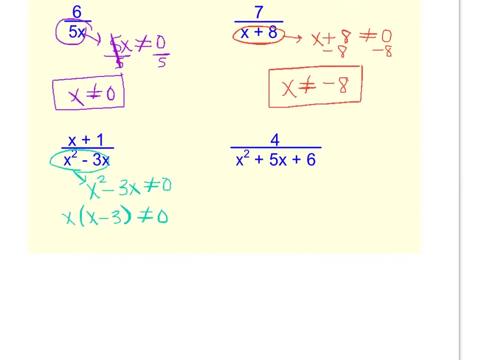 So we could take an x out of both terms and you're left with x minus 3.. So there's our equation. Let me make some more room. So now that it's factored, you're going to take your factors and say that first, x does not equal zero. 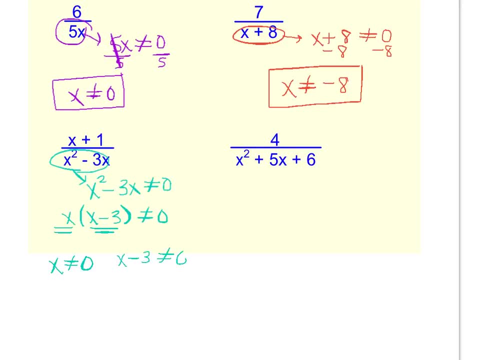 And the other, x minus 3, does not equal zero. Solve either of those for x to figure out what your excluded value or, in this case, values we're going to get. two of them will be. So the first one actually is: solve. x cannot equal zero. 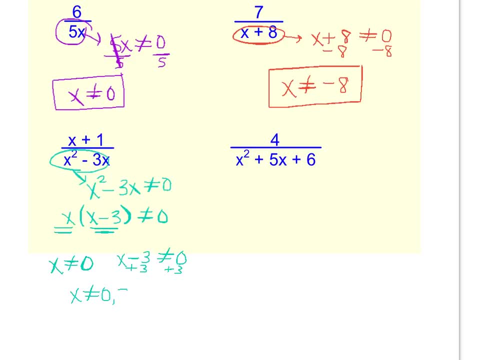 The second one. if you add 3 to both sides, you get a positive 3. So x cannot be a zero and a 3. Those are the two numbers that, when plugged in for x, would give you zero in the denominator. 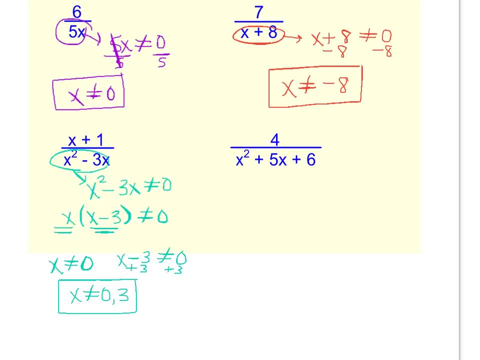 All right, our last example up here looks a little bit trickier. more going on. Go ahead and grab your denominator. So the entire denominator x squared plus 5x plus 6 cannot equal zero. So the entire denominator cannot equal zero. 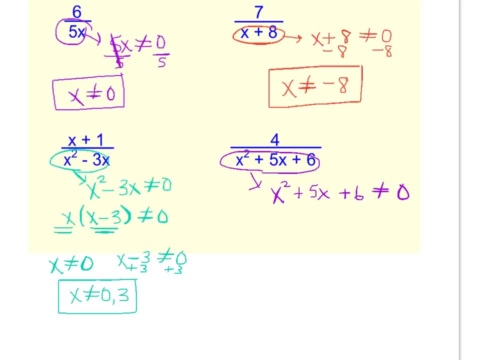 Now this is a trinomial, which means we're going to try to factor this. We want to look for factors of 6 that add up to your middle term of 5.. So it multiplies to 6 but adds up to 5.. 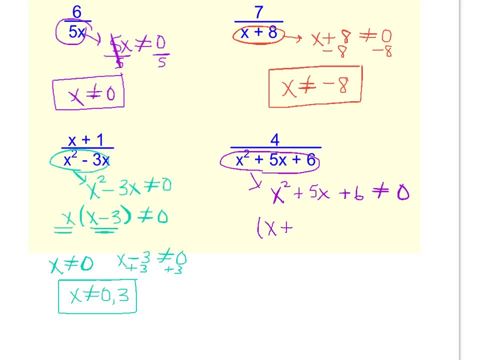 A positive 2 and positive 3 will be our factors. So we'll say x plus 2, x plus 3 does not equal zero. And then you take each factor and write those little mini equations. If you take each of those and solve for x, we'll subtract 2 on both sides. 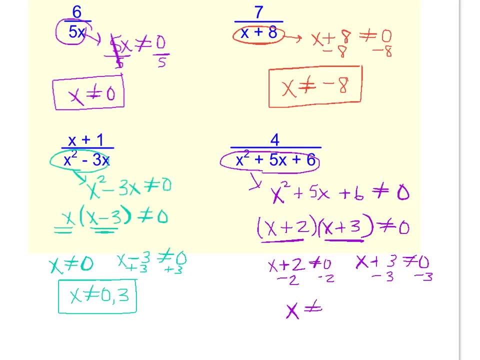 and then we'll subtract 3 over here. So in the end x cannot equal a negative 2 and a negative 3.. x can be any other value except for those two. Those are the two values that would make that rational expression equal.